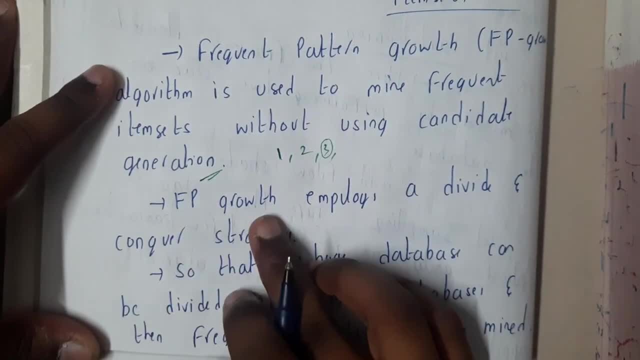 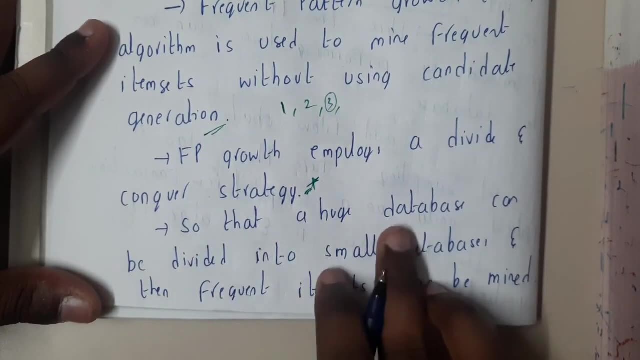 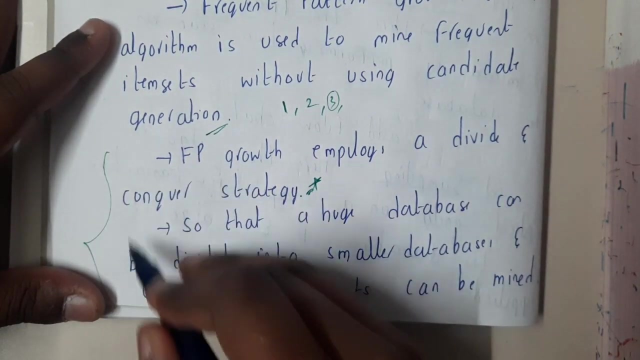 Yes, So those things will not be generated here. Okay, FP growth employs a division and conquer strategy, So this is also an important thing. Okay, So that a huge database can be divided into smaller databases and the frequent items can be mined. Okay, Yes, So. 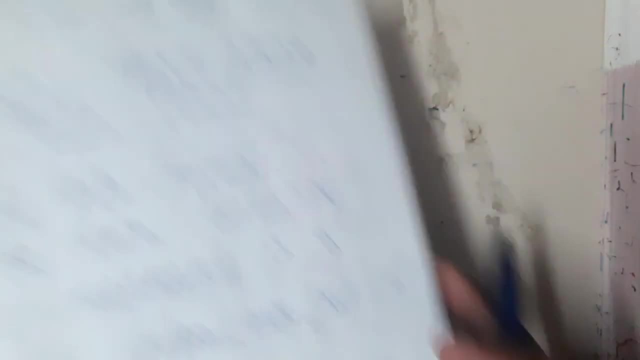 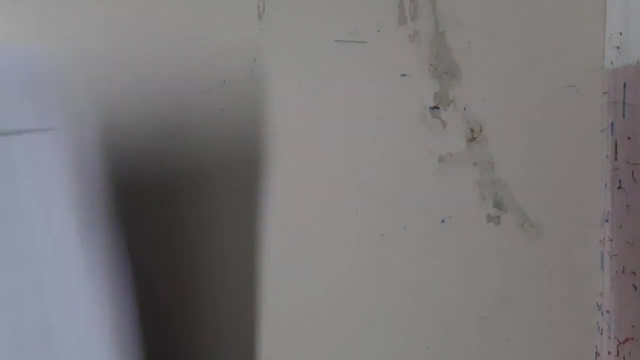 even if you do not remember these steps, it will be fine guys, But you need to have a clear idea about the algorithm, guys. Sorry about the process, how we are doing, Okay, Yes, So I hope everyone knows what to do. first step, right, Yes, So first of all, 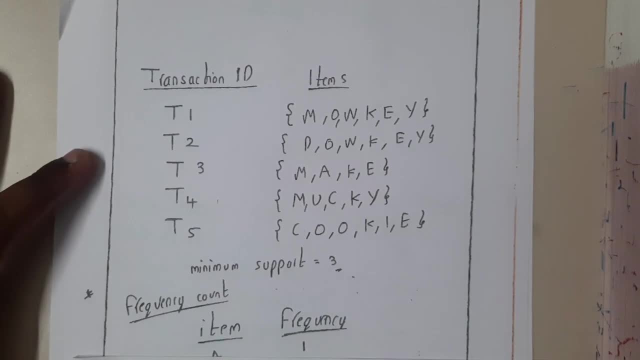 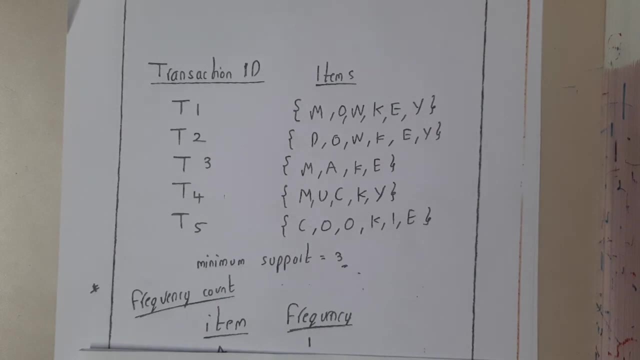 please take a piece of paper and here is a question, guys Okay, So I think this is also a previous year question or it is a textbook question, guys Okay, Because I forgot to add the question from where I have solved it and even now I was in, I tried to search. 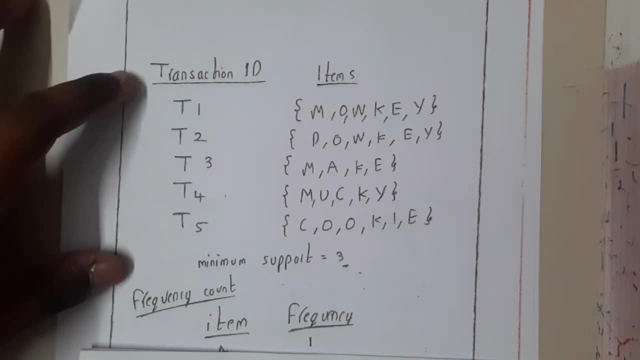 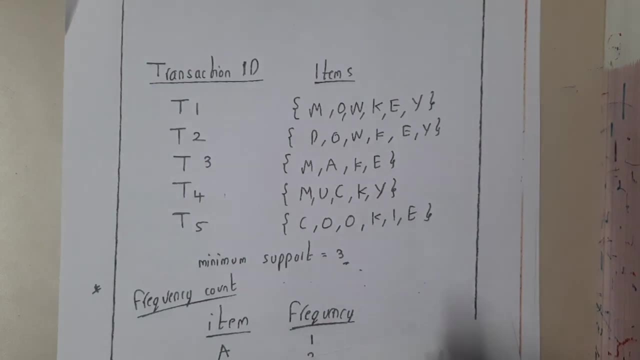 in the question papers, but I did not find it, guys. Okay, Okay, So let us see. So here we are having a five different transactions with five different words, right, Yes, So here we are having only a single. that is nothing but a minimum. 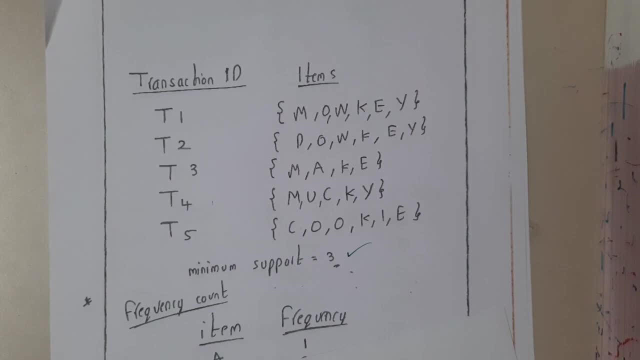 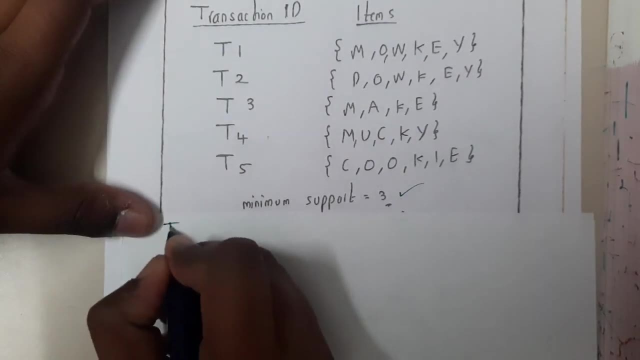 support. We are not having a confidence score. So in the next lecture I will be taking an example with confidence score, guys, Because most of you want with confidence score, right, Yes? So let us copy down the question: T1, T2,, T3,, T4 and T5.. Guys, I hope everyone also. 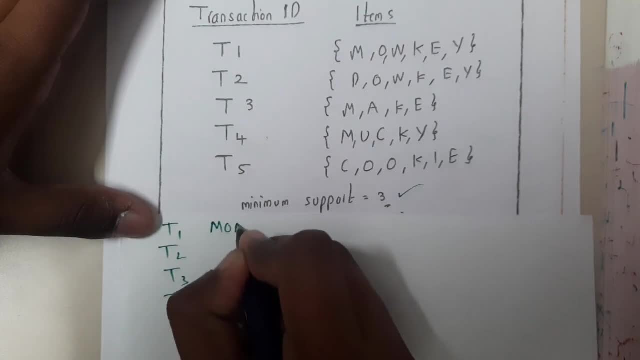 took a piece of paper, right? Yes, So write: monkey, M-O-N-K-E-Y, Donkey, B-O-N-K-E-Y, Make M-A-K-E, M-U-C-K-Y, Cookies, C-O-O-K-I-E- Okay. 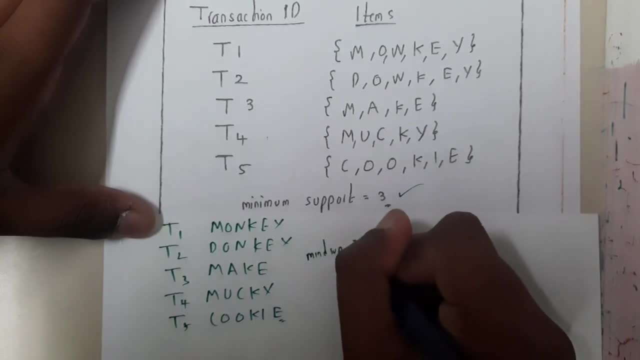 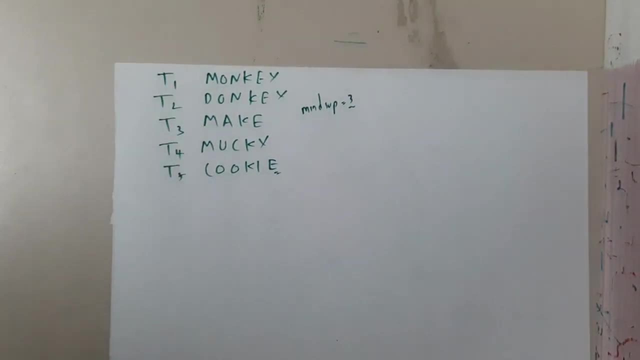 Yes, So minimum support count is equals to 3.. Okay, So I hope everyone remembers the first step of the normal approach, right? So the Apriori algorithm, So the same step we will be using here, guys, But only once we will be counting. 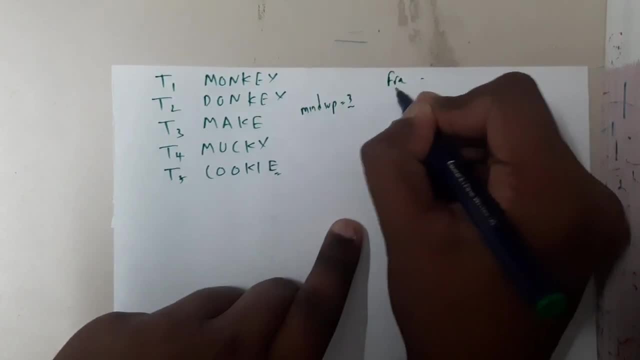 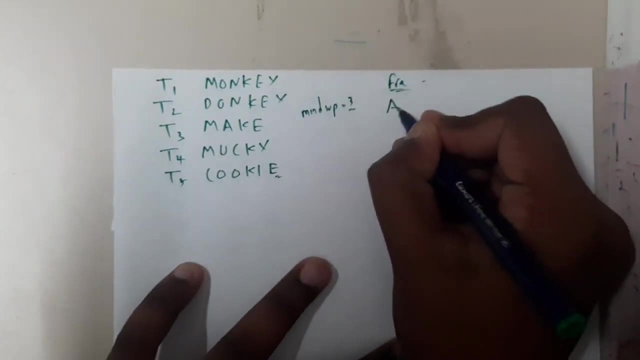 Okay, So now we will be writing the frequency count. Okay, So what are all the letters here, guys? Okay, So for this time I will be just copying the letters, guys, Because if I start identifying it will be taking few minutes for me. I am not that much fast. 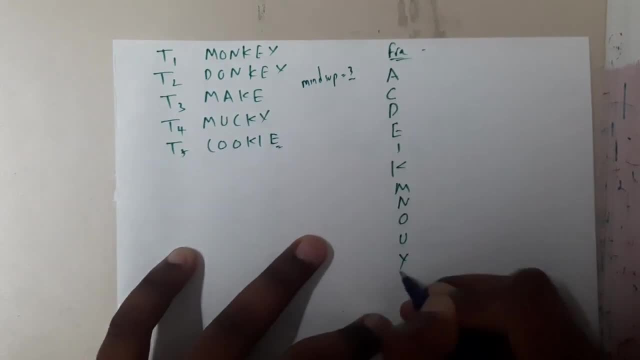 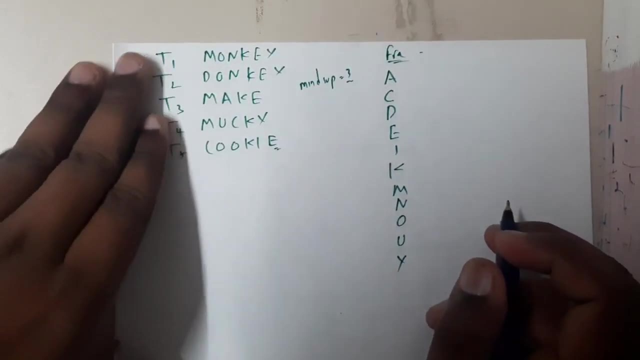 with alphabets. Okay, N-O-U-Y. Okay, Yes, So we wrote all the alphabets which are there in it alphabetical order, So it might be any order. It is no issue, guys, Okay, Yes. 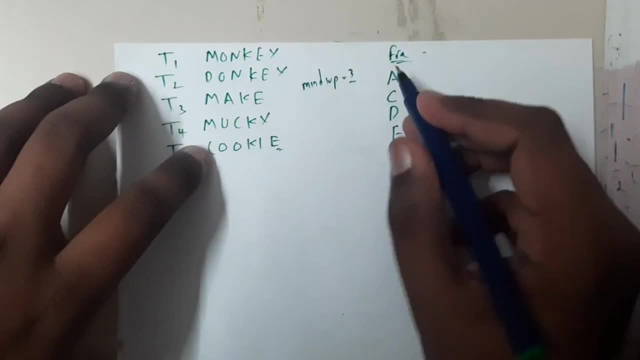 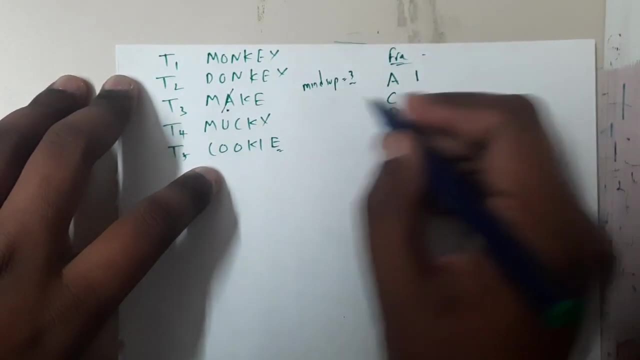 So now write down the frequencies: how many times Okay. So A Here, only one time I can find Okay Similarly. so I will be cutting it here, guys, Because it will be easy for us: C, One, two, Okay, D, How many times it is. 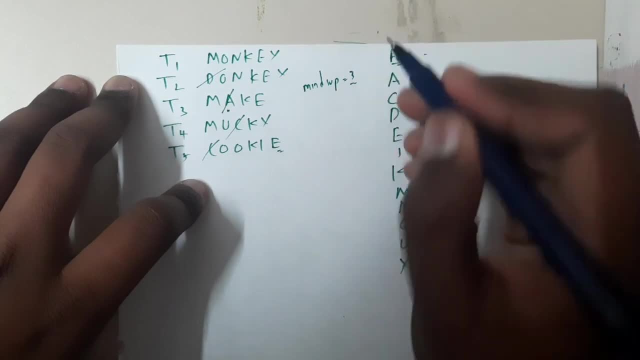 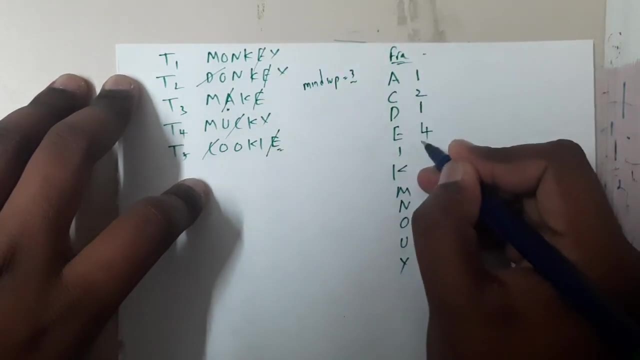 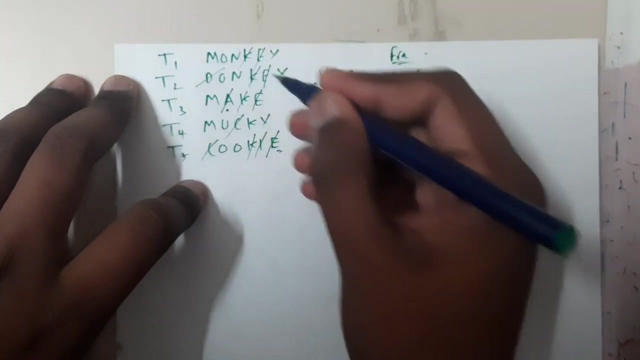 there One Okay. I think only once a day is there Okay E. One, two, three, four. Okay, E is four times Nice I. I is also one time Okay K. One, two, three, four. 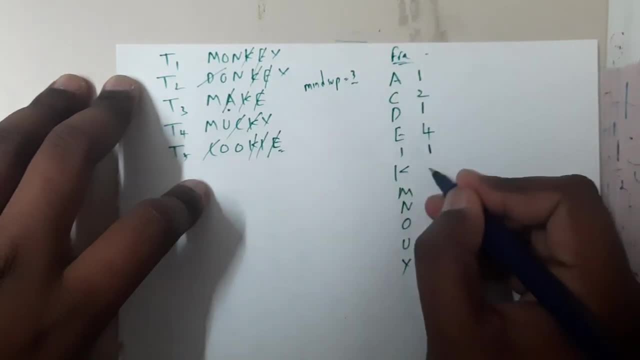 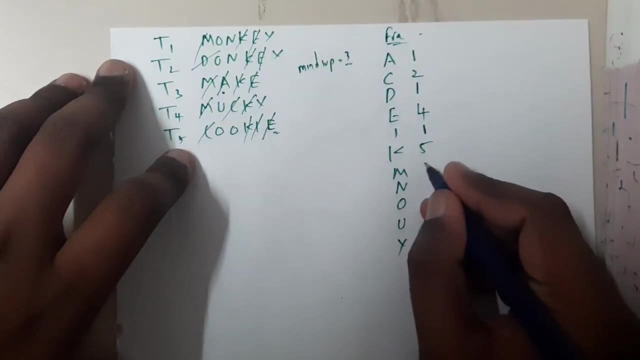 Four, four, four, Yeah, Five, Okay, In every letter it is there. Wow, In every word it is there. Sorry, M, One, two, three, Okay, I think it is three. only N, N is only twice. 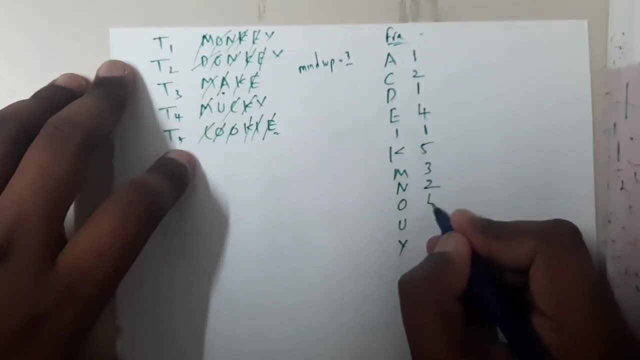 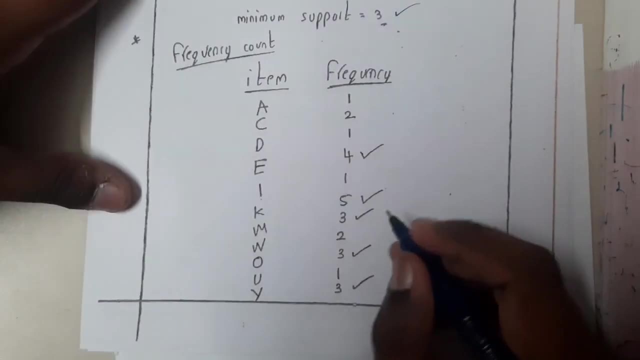 Yes, O, One, two, three, four, Wow. O is four times Okay, But I think I wrote in the book as only three times Okay, So here I wrote only three times. guys. O is four times I. 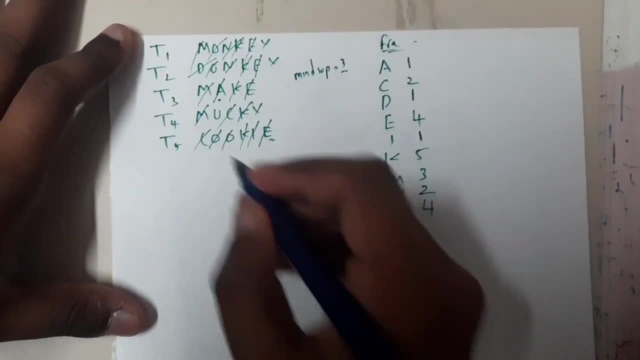 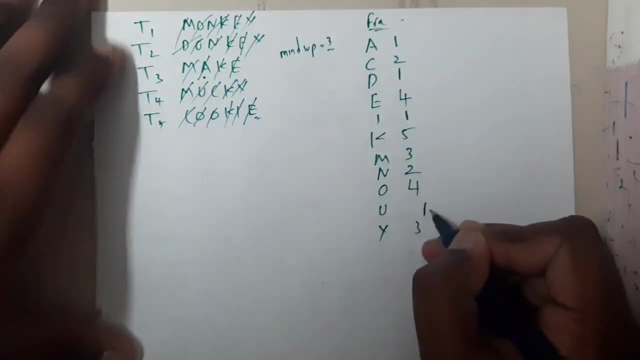 updated it. Nice, Okay, U One Only once, right, Yes, Similarly Y One, two, three, Three times Okay. So I found a mistake in my paper. now, Okay, Let it be for now. It is fine, You can manage. 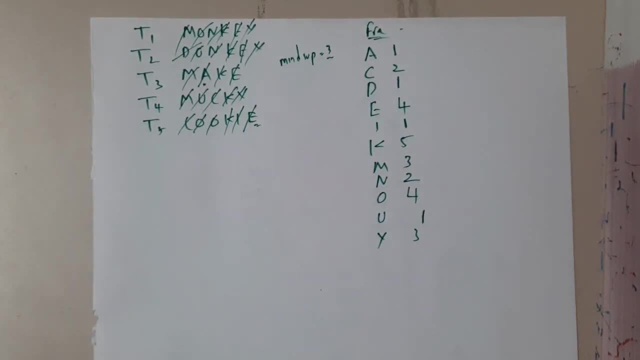 Okay, So now we got these values right? Yes, So now our minimum count value is three right guys. Yes, So now you need to identify: wherever we got the value less than three, we need to cancel it because they are not allowed to the next round, right? Yes So. 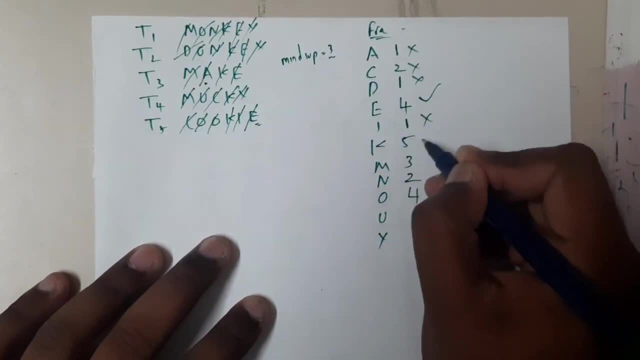 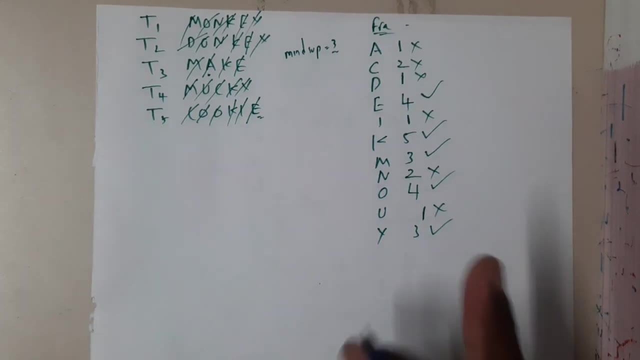 just cancel them. No, no, no, Yes, No, Yes, Yes, No, Yes, No, Yes. So now the first thing that you should do is you should write in ascending order, guys, Sorry, Ascending or. 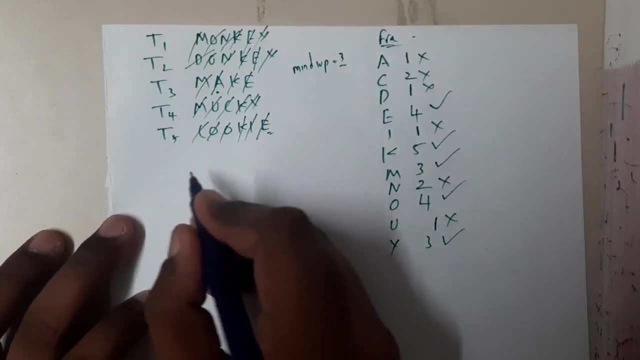 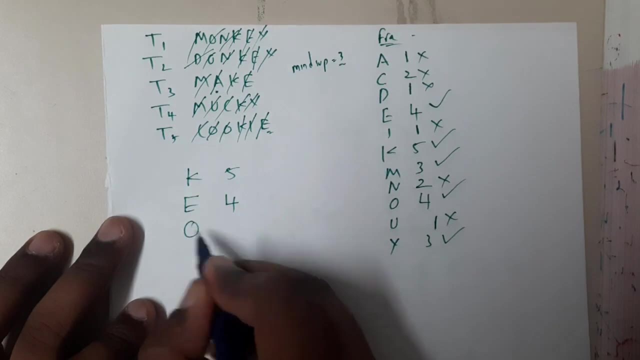 descending, Sorry, Descending order. So like maximum to minimum. So what is the maximum? K? we are having five, Then we are having E, four, Then we are having O, also four, I think in example I wrote with three only. 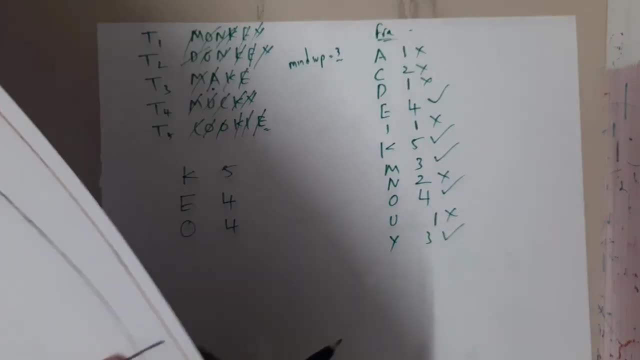 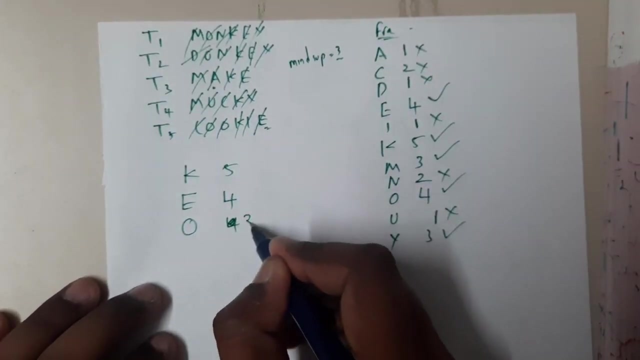 Okay, Just let me cross check it once again, guys. Cookie double O? right? Yes, I think it should be taken only once because it is in a single line, right? Yes, I think that's the issue here which I am doing wrong. Okay, Yes, Yes, guys, It should be taken only once. 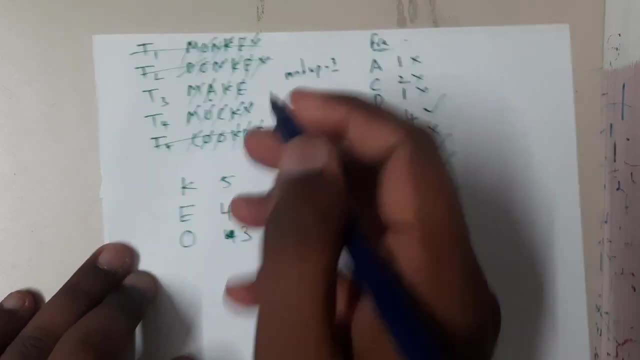 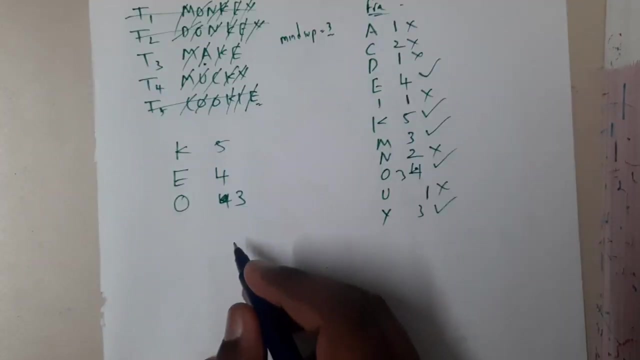 because how many, in how many transaction it is occurring, is the question right, Not the count of exact count, right? Yes, Now I got the point why I wrote three. Okay, Yes, Because while I am solving it, I will be solving it from a book or from a website. So I am solving. 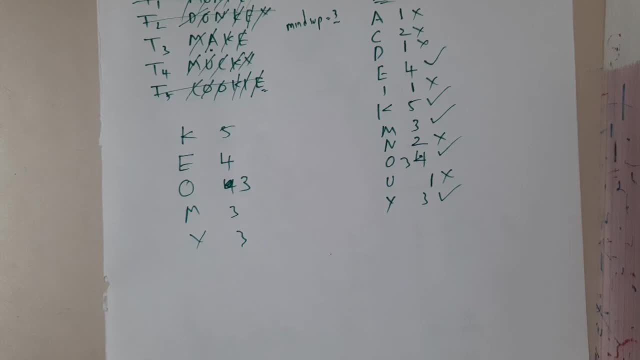 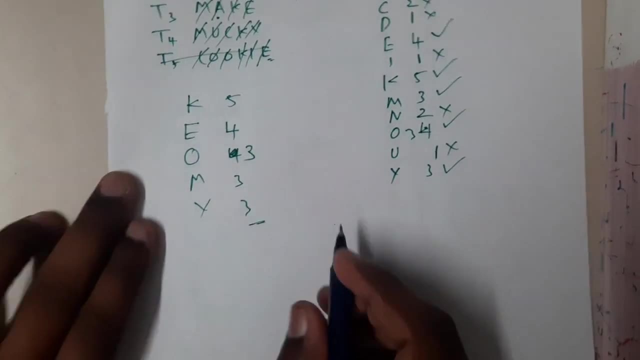 it from a website, right? So that is the reason why the question going wrong will be really rare, right? Yes, And that I myself identifying is a bit funny, Okay, So let us continue. Okay, So now you got the order right. Yes, So here I wrote M O Y, So let. 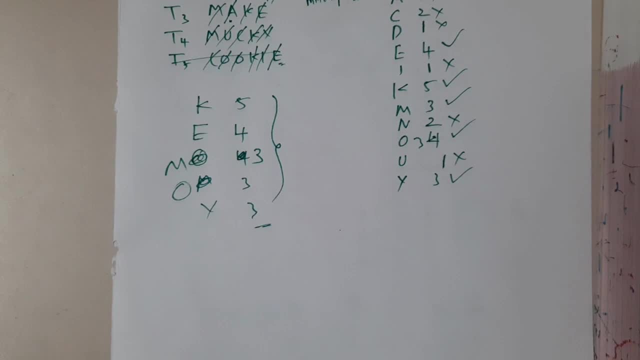 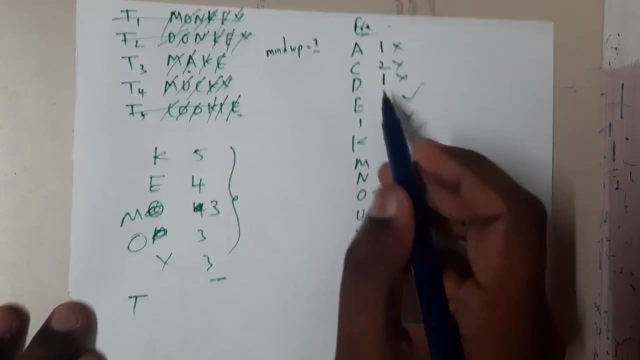 me change it, It will be better for me. M O Y, Okay, So K E M O Y. So basically in this order, arrange each and every transaction, guys. So rest all letters like A, C, D, I. 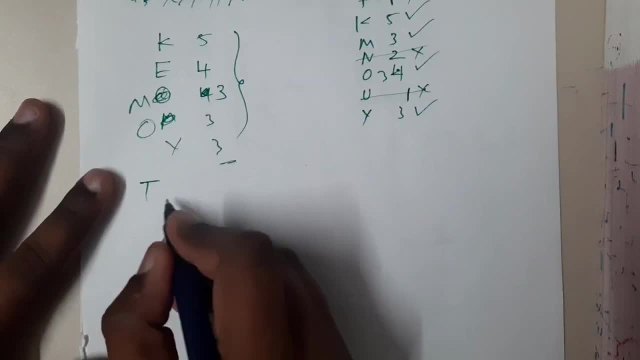 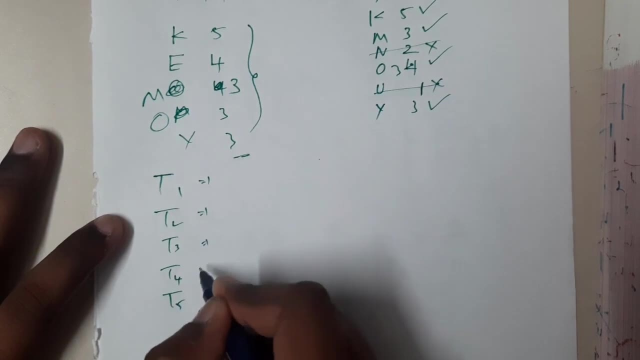 and U Remove them. There is no use of them. They are useless. now, Okay. T1, T2, T3, T4 and T5.. Okay, So I will be directly converting them, guys. So it will be K E M O Y, Okay. 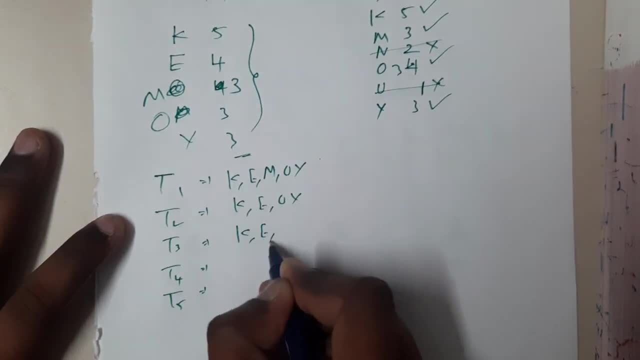 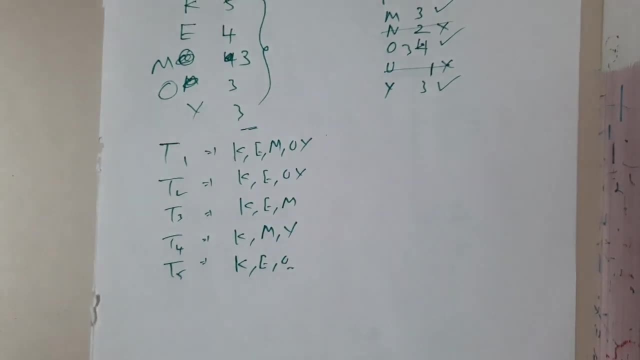 So K E O Y Okay. So K E M Okay. So K M Y Okay, So K E O Okay. So you might be having a doubt that. So how did I do it that much faster? I have just copied, I have. 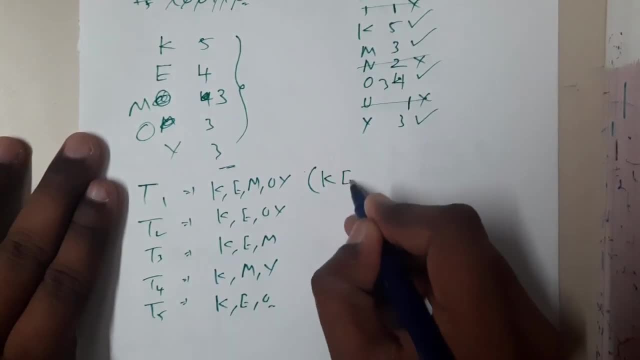 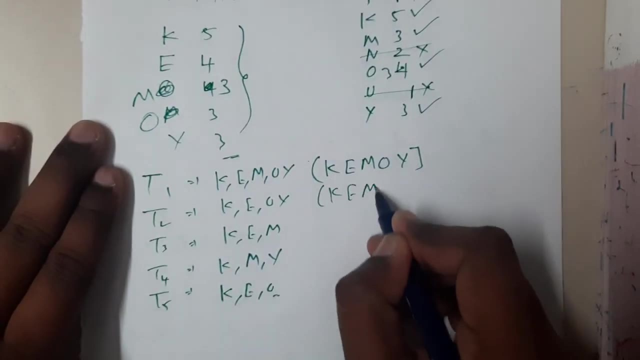 copied them. So let me say you how I am, how you can do it in examination. first, Okay, Take pencil, guys in examination and write this five, six, five times. Here we are having five transactions, right? Yes, So write it five times, Exactly The exact text you write. 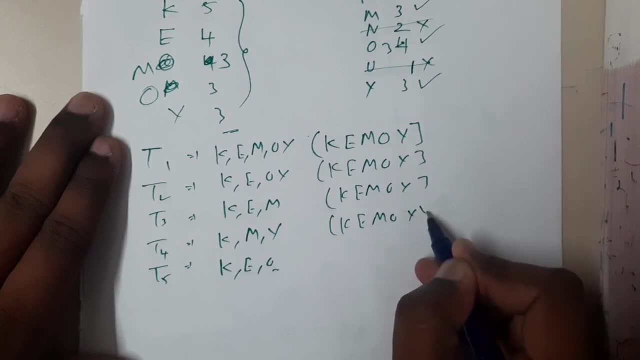 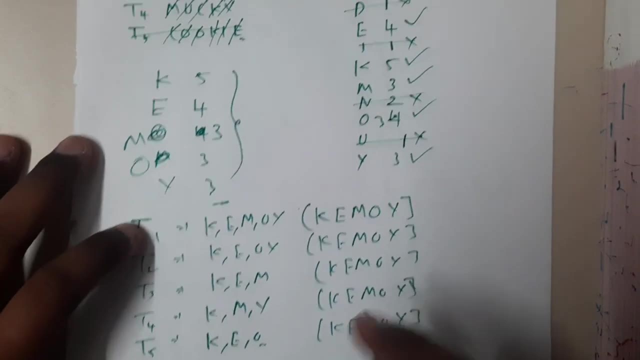 it guys. Okay, So K E M O Y. Okay. So, K E M O Y. Okay. So, once you wrote it, So take the first transaction. The word is a monkey, right, So M O N is not there, K E. 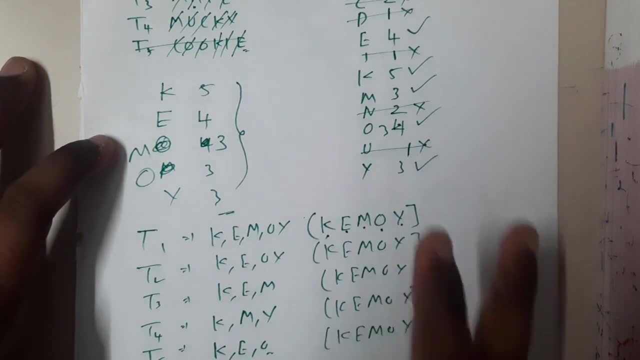 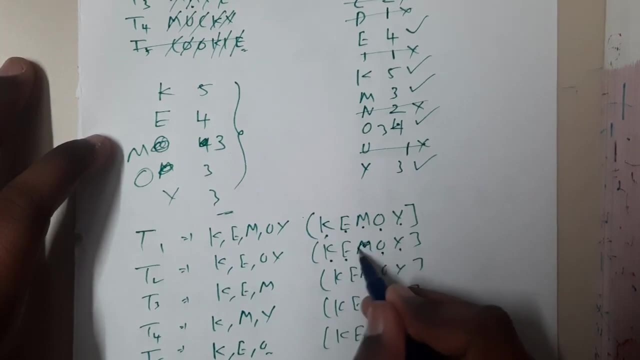 Y, So every letter is there, So all will be coming here. The second letter is a donkey, So D is not there, O N is not there, K E Y M is not coming, So remove M, So this. 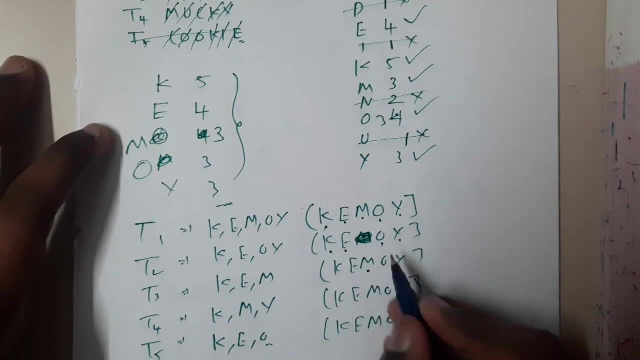 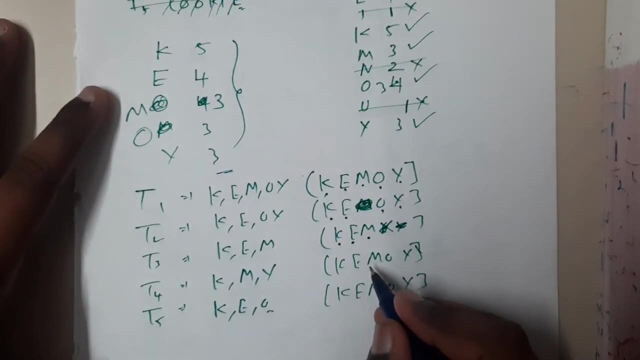 will be the result. The third one is a M A K E M. A is not there, K is there, E is there. So remove these two. Done Similarly: M U C K Y Mu key. M U C K K E M O Y. Okay. 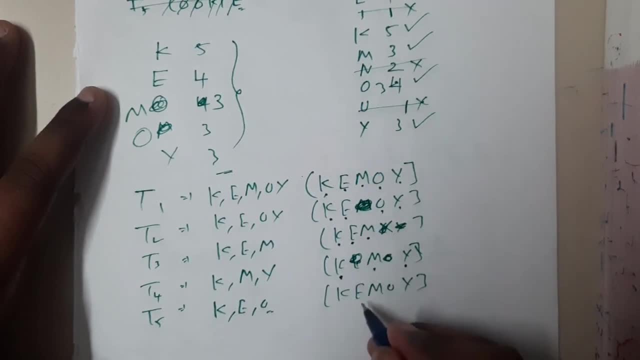 So these two will not be there. Okay, At the last cookie. So O will be there, C is not there, K will be there, I will be there, E will be there. So at the end you will be. 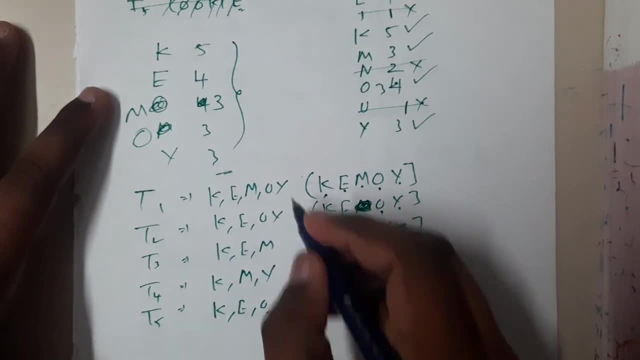 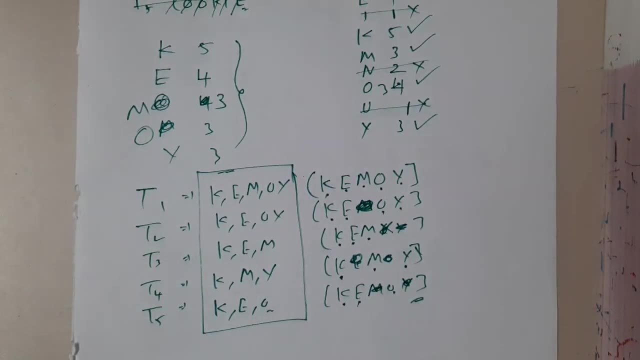 ending up with only these three, Okay, Yes, So at the end you will be ending up with these things, guys, Okay. So, once you got this, almost your problem- 90%- is done, guys, It might be sound, sounds a bit funny, but almost 90% of your problem is done, Okay. 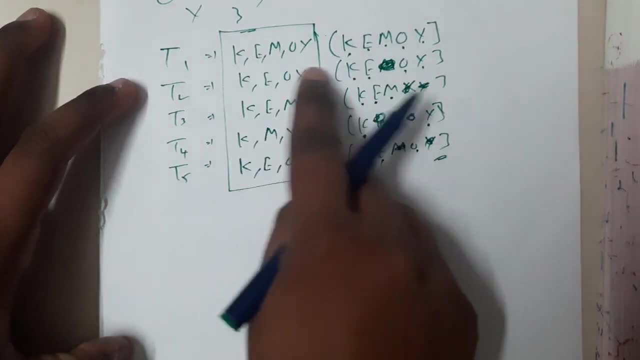 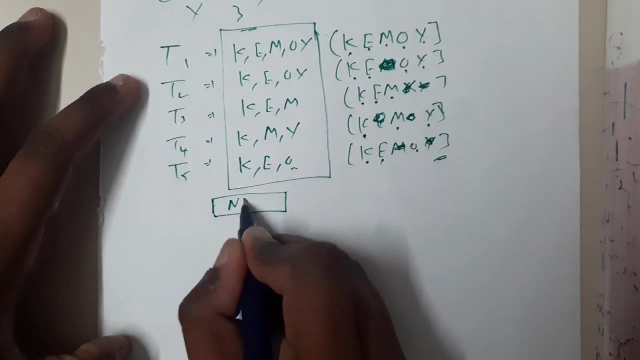 Yes, So now your only step left is you need to use these and form the transaction. So start a tree, guys. Okay, Yes, So please concentrate now, guys. I don't know how many of you took the paper and solving. You are solving, But if you did not take, please take. 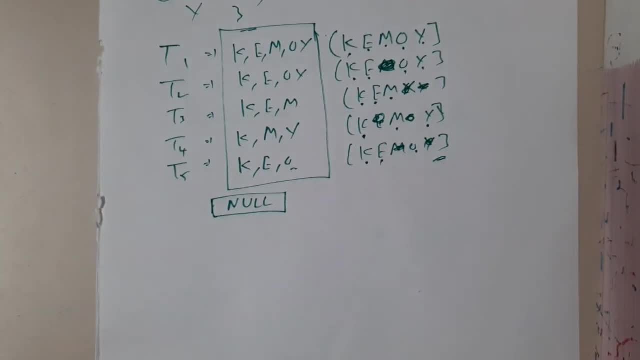 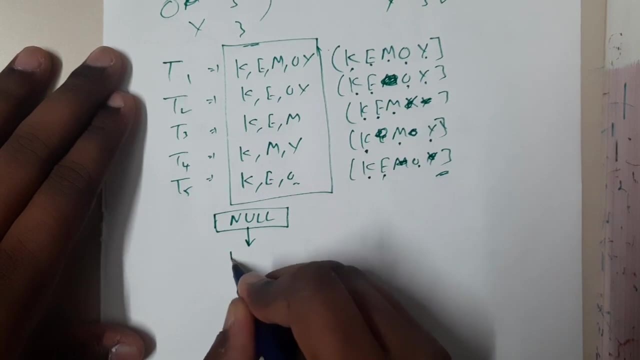 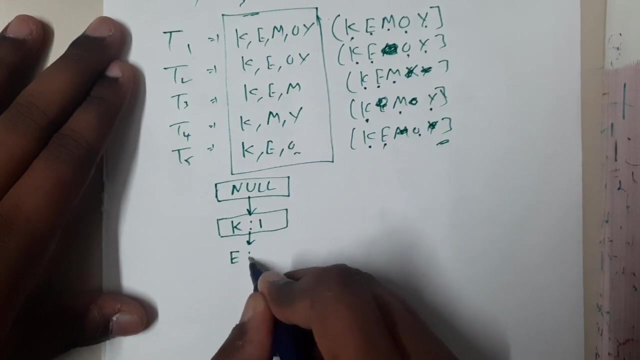 at least now, guys, Because from here you need to concentrate, because this is the important thing. Okay, Yes, So the first word is nothing but K E M O Y, Right, Yes, So start it. Okay. So K colon, how much time One time? Okay, Like step by step. K E is also first time. 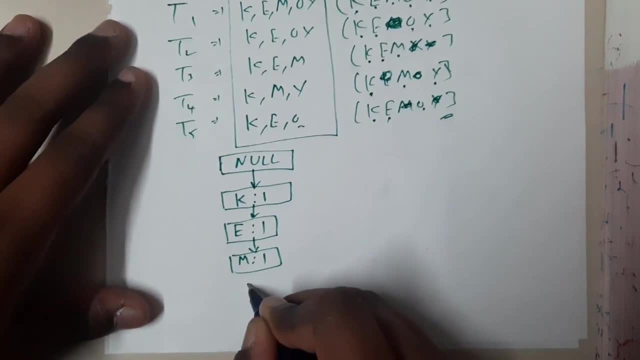 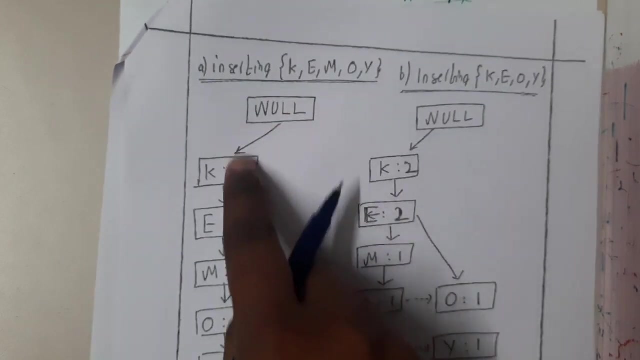 M is also first time, K E M O is also first time, Y is also first time, So you wrote for this, Okay, So this will be your first step, guys. So A inserting the K E M O Y, you will be inserting them. 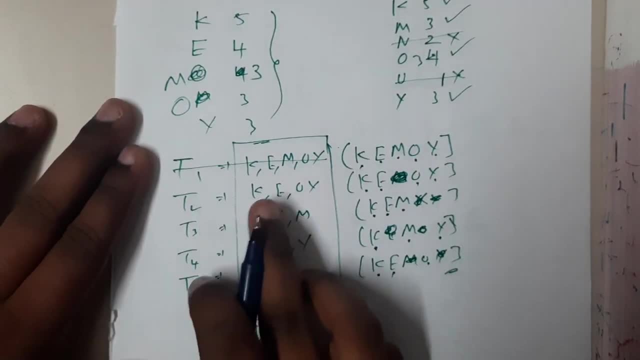 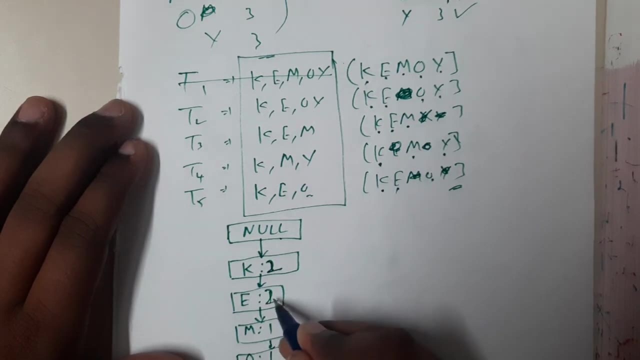 Okay, So now this insertion is done. So now insert the second one: K E O Y. So from here you can go to K here. So you just increment it. You can go to E also, but you cannot go. 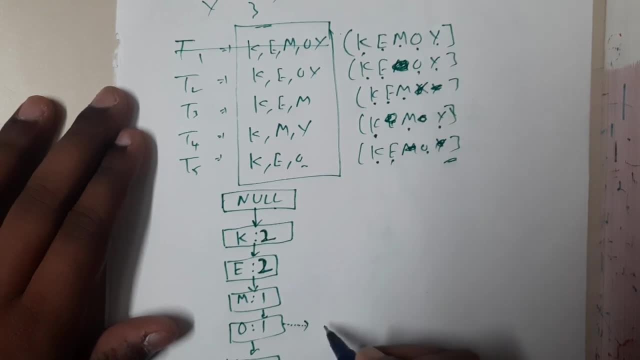 to O guys. So let us make a dummy pointer here. Okay To O, colon 1.. Okay, So from E I can directly go to E by bypassing M. So that is the trick here. Okay, So I bypassed it and went to. 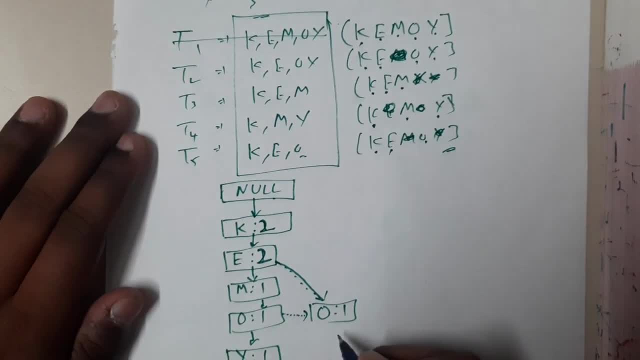 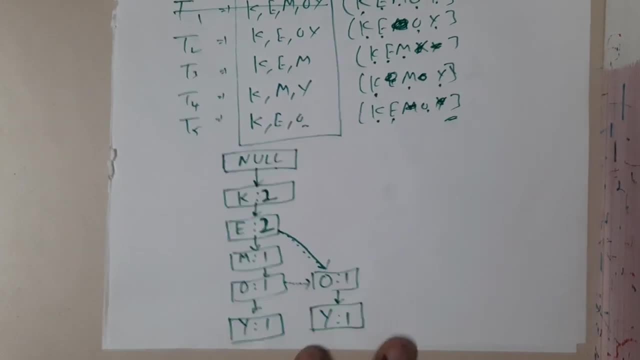 O. So after O again, I need to go to Y. So instead of making any confusion, let us make it down only. Let us make one more duplicate for Y. also Done, Yes, Okay, Yes. So now. 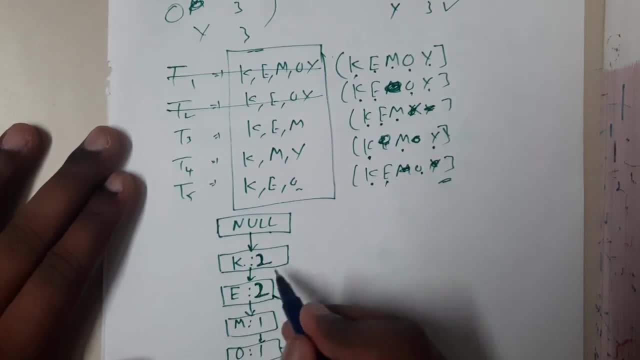 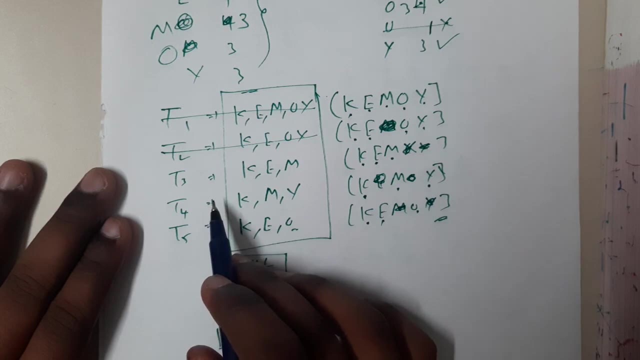 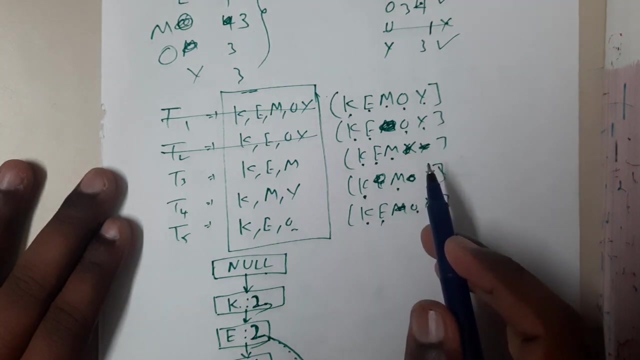 you are done with the second one, So continue in the same way, guys. So K E again, it is common 3. Okay, So after K? E, what is there? Okay, Just give me a second, guys. Okay, I think, okay, let. 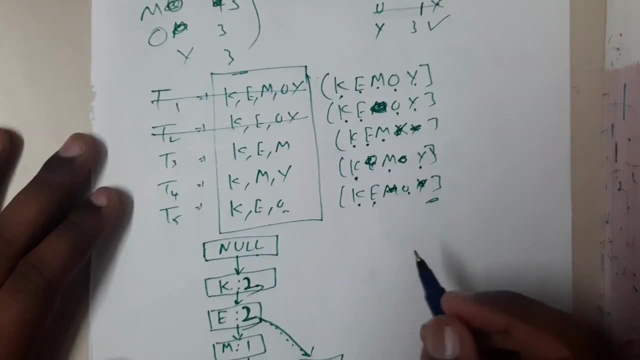 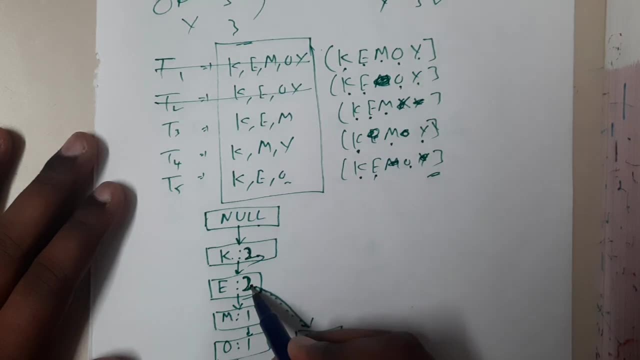 it be for now. There is no issue. Okay So K E. after that we are having directly M So K E. Okay, So from K? E you can go directly to M right. Yes, So here. directly to M means. 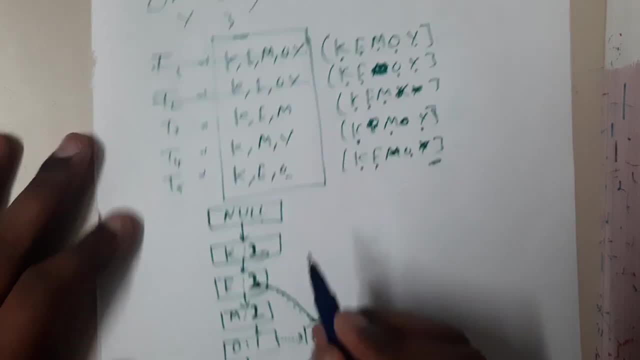 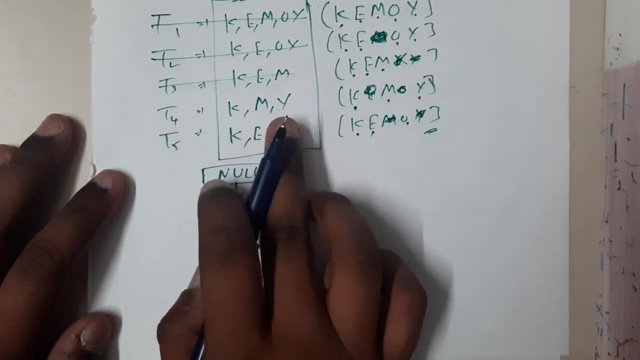 here the increment will be 2.. Right, Yes, Again. here, only you will be stopping. So K E M. So it is already in order. K E M, It is fine. The next one is K E. sorry, K M Y. Right, Yes, So K M and Y So they. 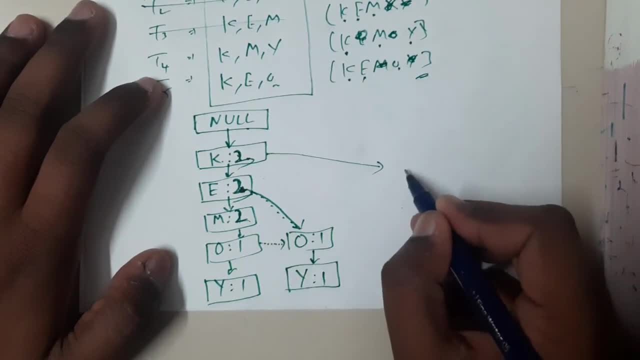 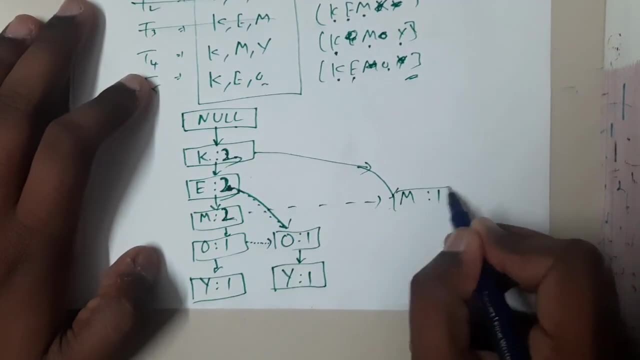 are almost alternate. So from K you can directly create one dummy to M. So till here it should come. So to M, colon 1.. So it will be pointed in this way, Okay, Okay, Just give me a second. I will return in the paper. 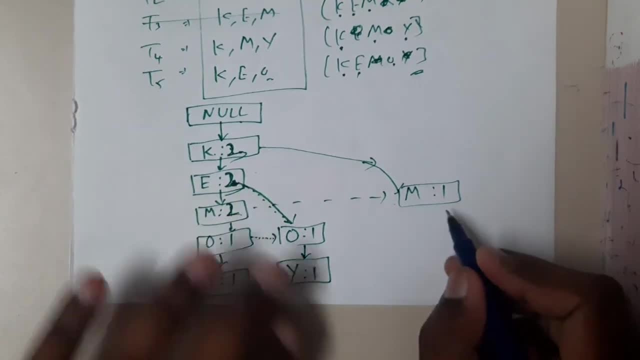 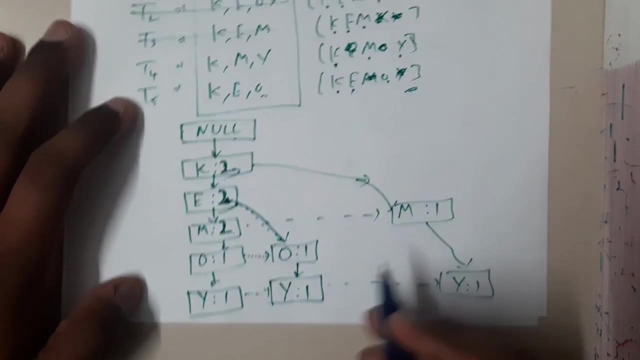 Guys, Okay, M from M you can directly go to Y, colon 1 again, Right, Yes, So again, these are all our pointers, guys, dotted pointers, Okay, So now we are done with this also. 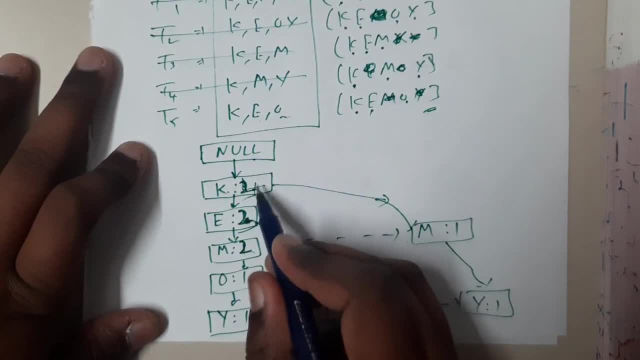 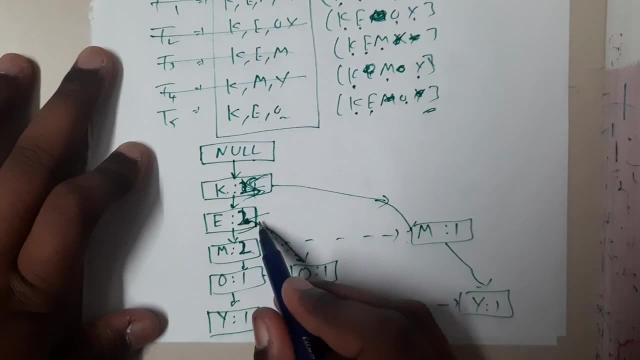 and the last one is K E O. So again, increment: This is 4.. Now this is 5,. guys, Everyone is starting with K, So 5,, 4 and O Directly from here. you need to go to O So you can. 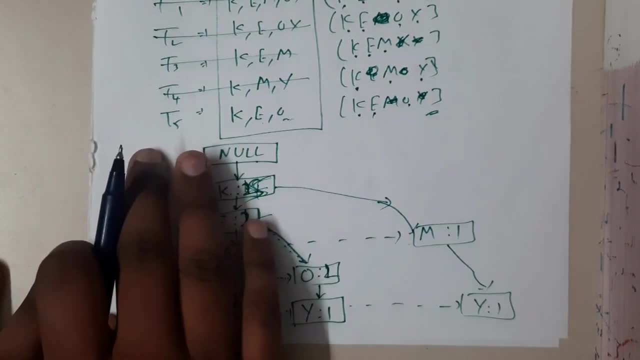 directly go to here. Okay, Yes, So at the end you will be getting the diagram like this: guys. Okay, Yes, So the next one is K E O, So you can directly go to O, So you. 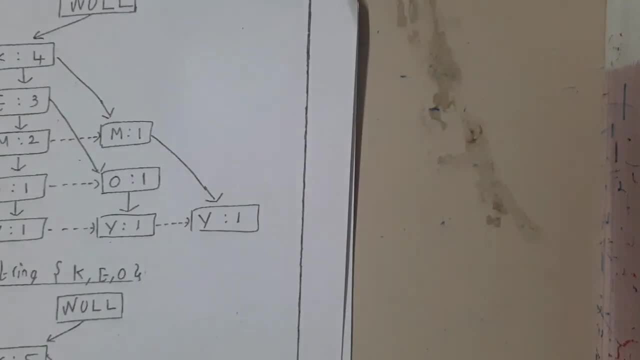 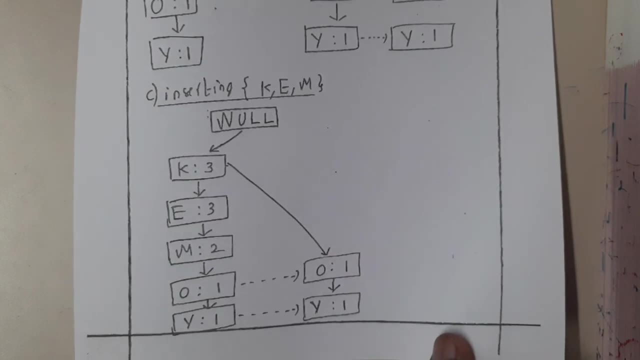 need to check this. This diagram will be in this way, guys, So please solve it step by step. guys, In examination, you need to explain how you are doing it Right, So the steps will only showcase you that you are solving it truly Right. Yes, Okay, So once. 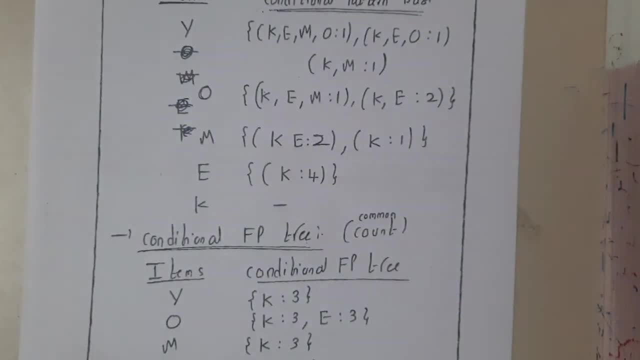 you solve it. you will be getting in this way, guys: Okay, Yes, So once you got that, So I will be continuing it on the next page. guys, Just give me a second. Okay, So now. 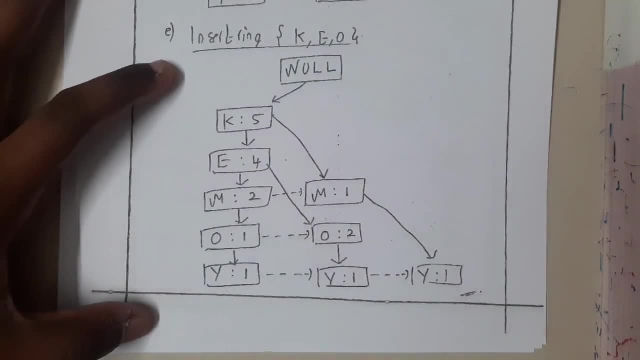 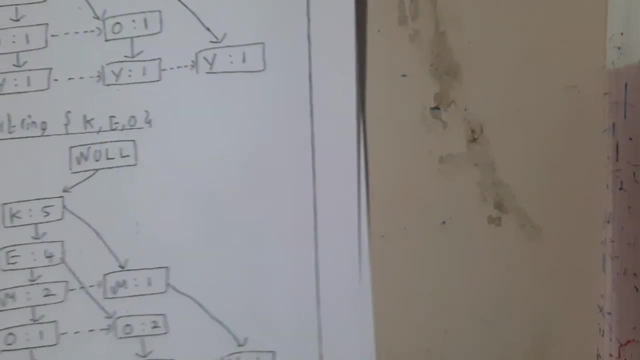 we got this Right. Yes, So assume that this is our final diagram, but this is a bit wrong. more letter x: okay, it's correct. only sorry, it is correct only guys, because we removed that o. right, yes, so this is correct. only so we will be getting in this way, right, yes, so once you got this, you 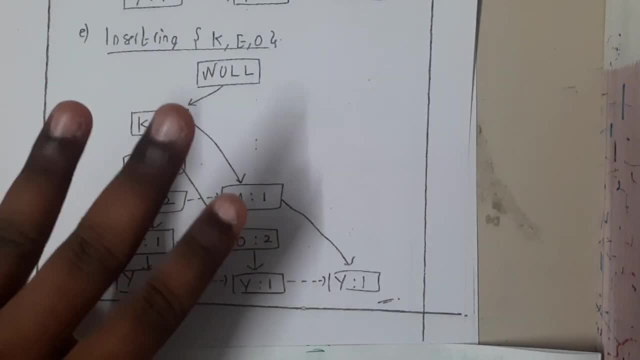 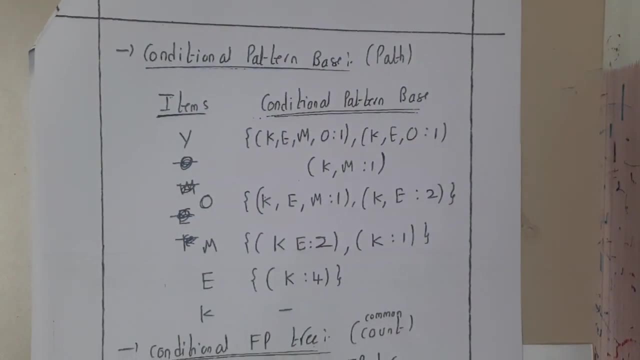 will be filling three different tables or a single table. three columns you will be filling, guys. so the first column is nothing but the conditional pattern based guys. so what is the path? you can say: okay, so the first step that you will do is you will be writing the letters in the reverse. 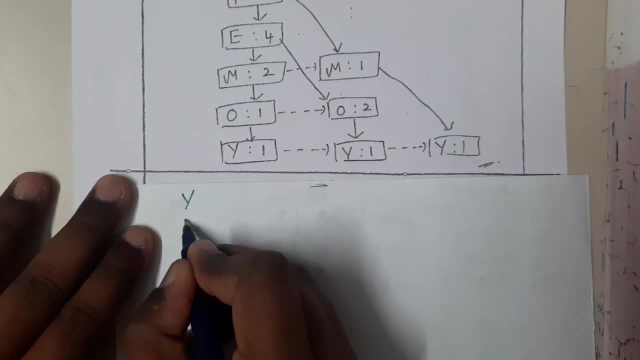 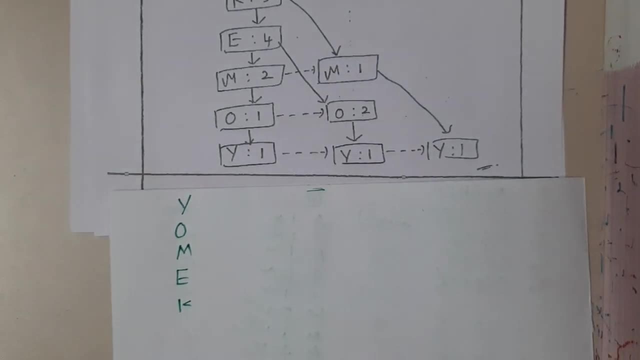 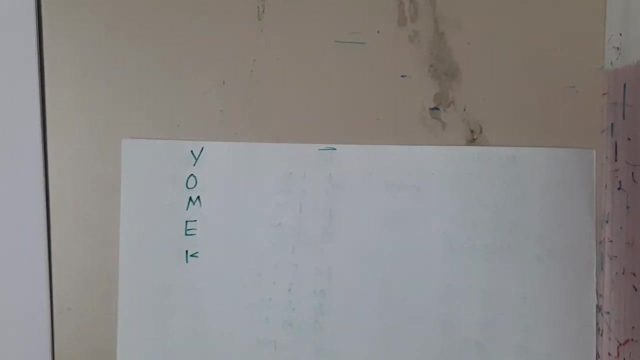 order guys from bottom to top. that is nothing but y, o, m, e and k. okay, so once you wrote them, you'll be starting the process. okay, so you will be doing the possible paths to the top guys. okay, so how many ways can you reach to y? so there are three different paths here. right, so to y. 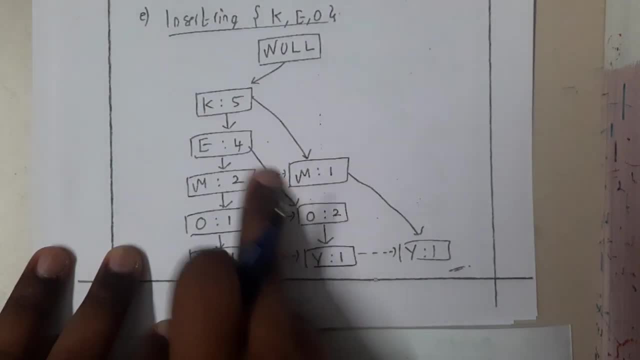 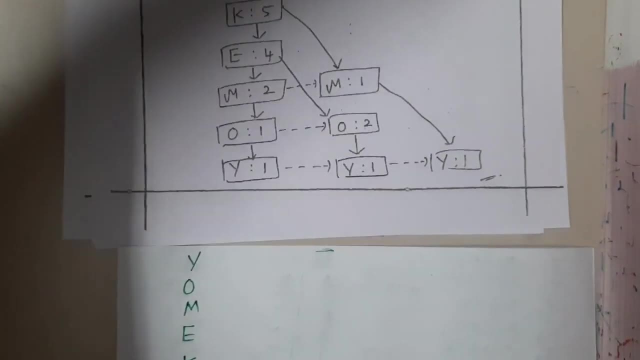 okay, so via this path, via this path, via this path. so now write those paths clearly here. that is the main thing here. okay, yes, just give me a second. i'll be opening the paper, guys, because i can cross check while i'm writing. okay, let me remove the paper. that will be better, right. 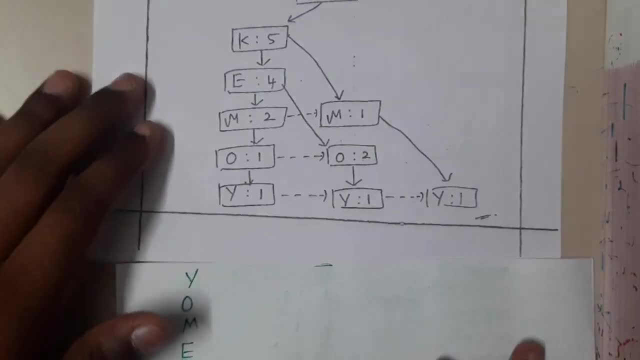 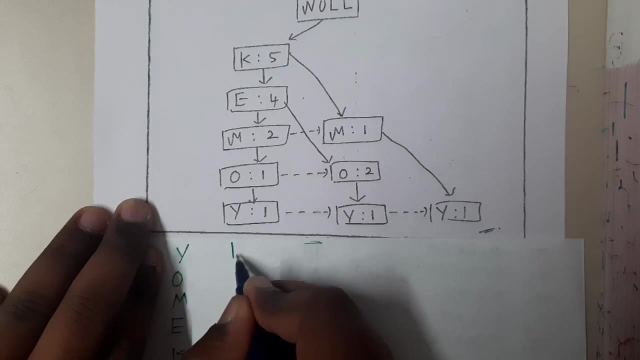 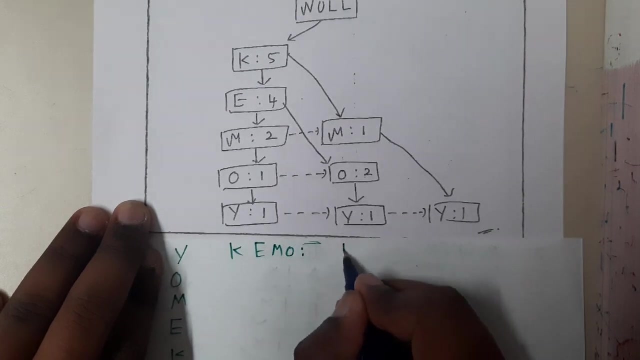 yes, okay, so now we got that. okay, yes, so now you are trying to reach y. in how many paths is the question? so you can start at k e m o and you'll reach y. okay, this is one path. similarly k e o. this is one path. similarly k m. this is one path. right, yes, so if you observe at all the last, 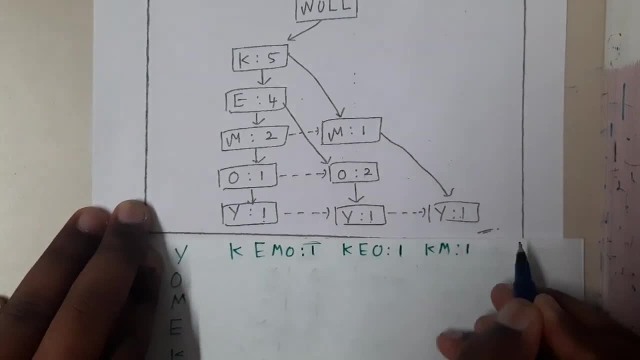 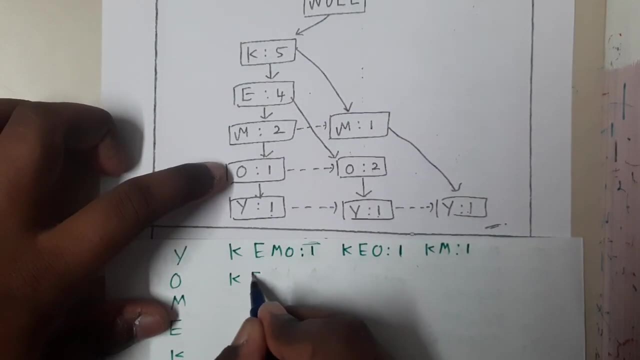 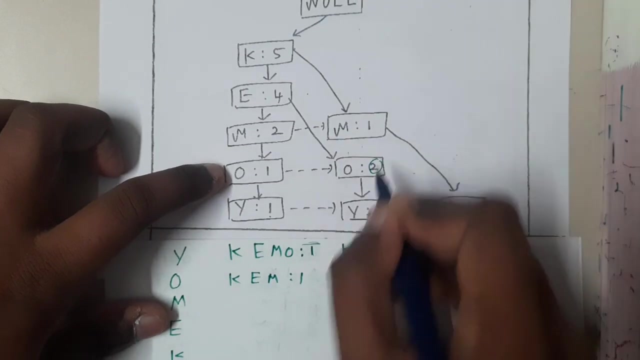 stages of y, it is one only. so there is no change here. so colon one. okay, so now do for o guys. okay, so for o. how many ways can we go from k e m, colon 1, k m, colon 2, because it is 2 here, right, yes, so 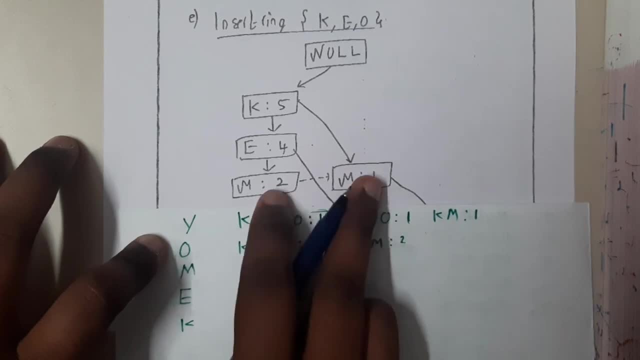 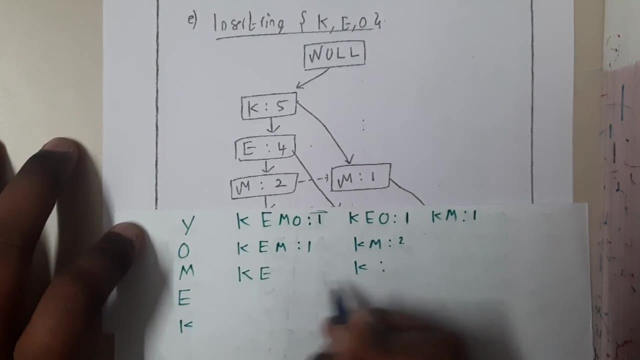 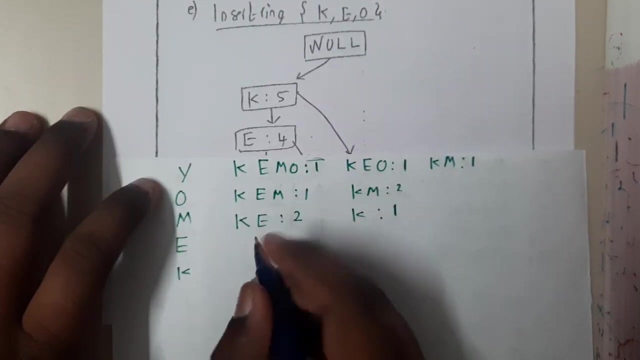 to m: how many ways can we reach? we can reach only in one, two ways, okay. so directly from k, you can reach, or directly from k e you can reach. okay. so in both the in this case it is two, and in this case it is one, okay. similarly, e so to e: how many ways? only one way is there. 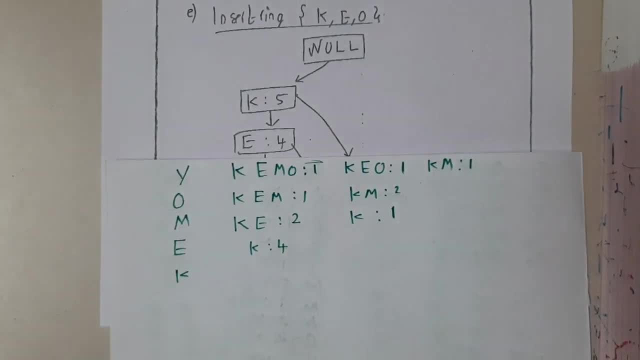 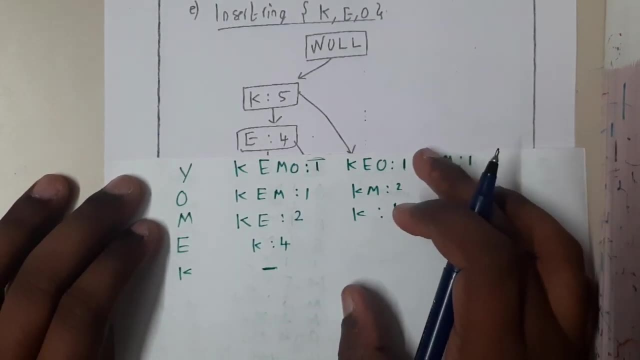 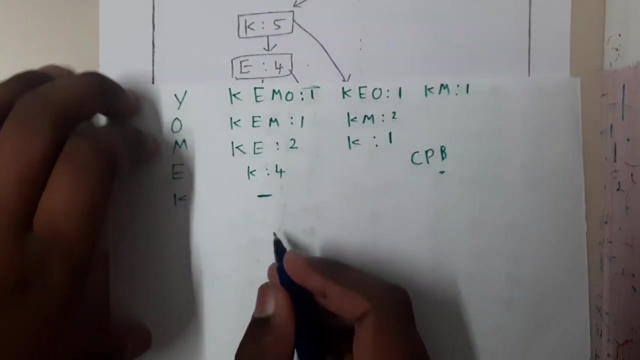 and that is nothing but. k e, k, sorry, k 4, right, yes, okay. and for k there is no path because it is at the starting point, right, yes? so this is the first table. that is nothing but conditional pattern base, guys. so, conditional pattern base, okay. and the second table is a nothing but. 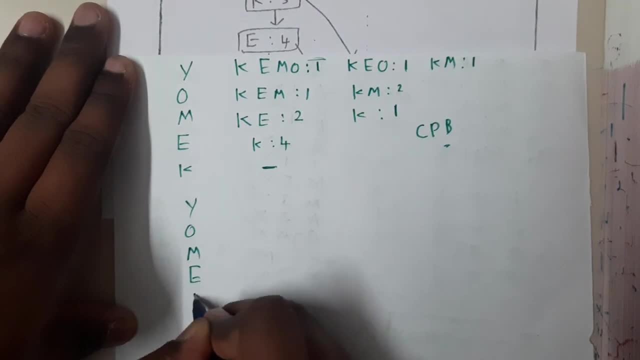 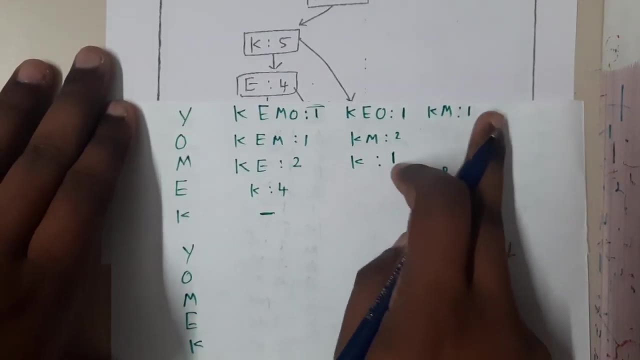 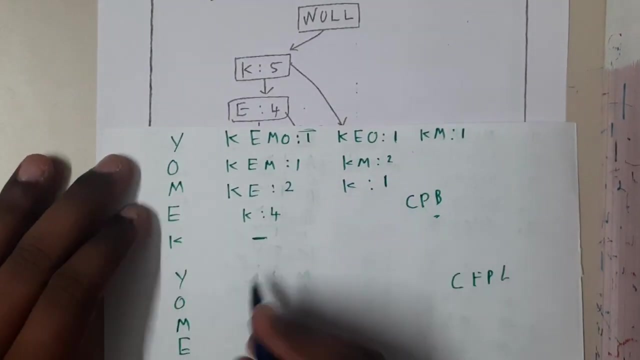 the same values. you write again, guys, okay, so once you wrote here, you will be finding the conditional fp tree. guys, okay, so you calculated here, right? so what are the common things here? so that is what you will be identifying here. so here, how many times k came three times. 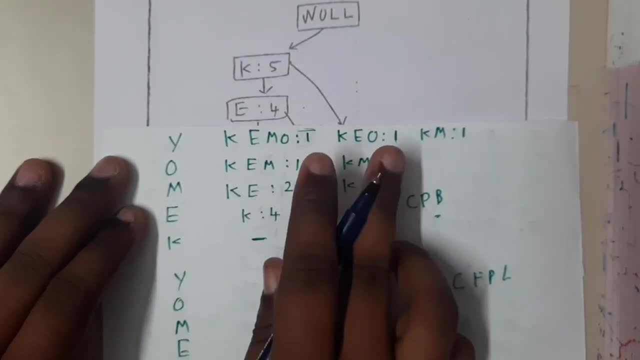 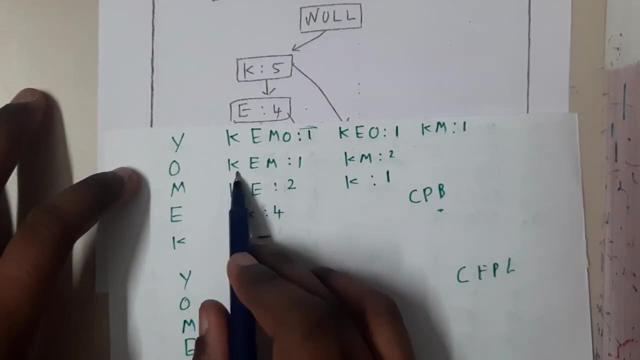 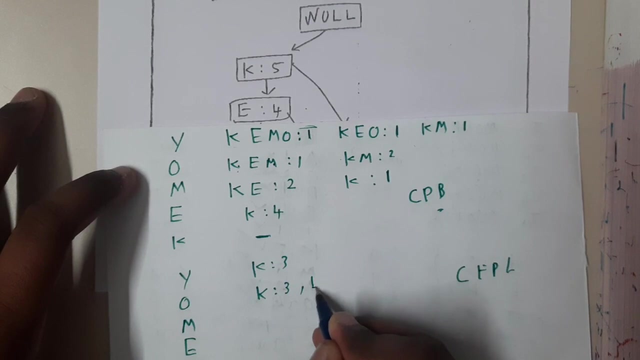 so e came two times, m came two times, o came two times. which is maximum k? how many times? three times. so that is the answer there. that's it. similarly, o in o. what is the maximum time? so k came three times, m also came three times. so here we are having two things: k and e also. 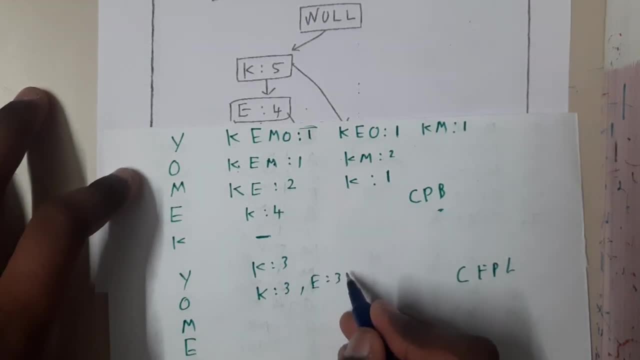 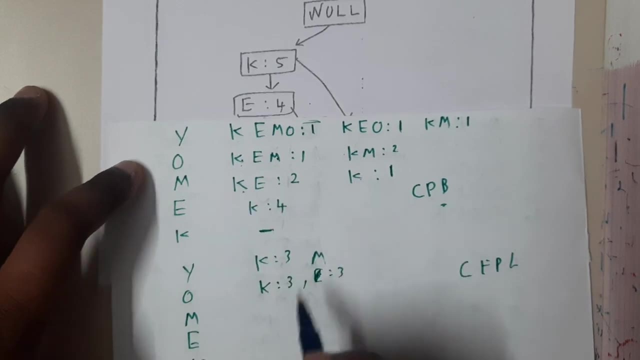 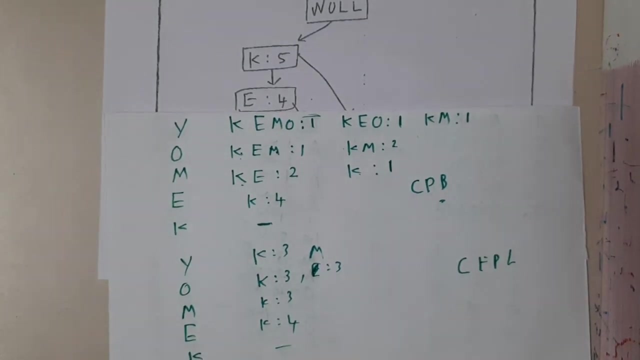 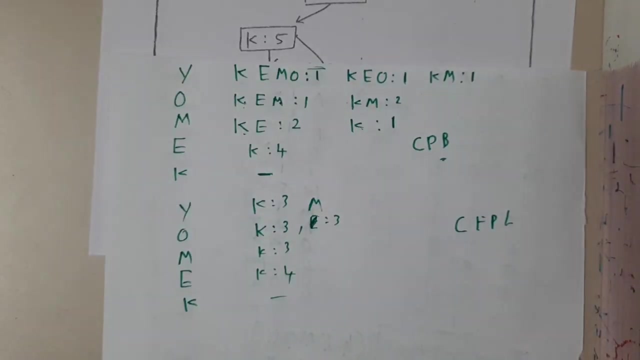 three times. okay, sorry, e or m guys. i think in paper i wrote okay, yes, sorry for that, okay. similarly, m in m k came three times. okay, in e k came four times and at k dash, okay, yes. so basically here i wrote e as guys. it is m really okay, sorry, it should be e only. 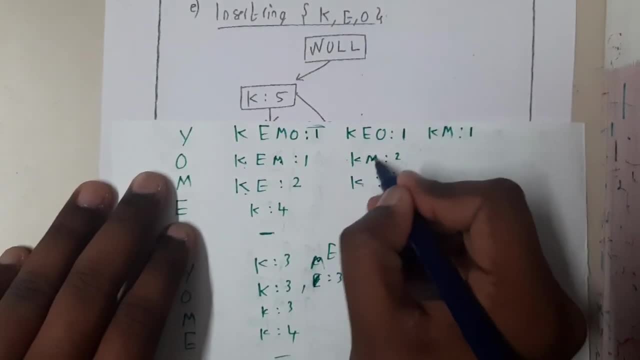 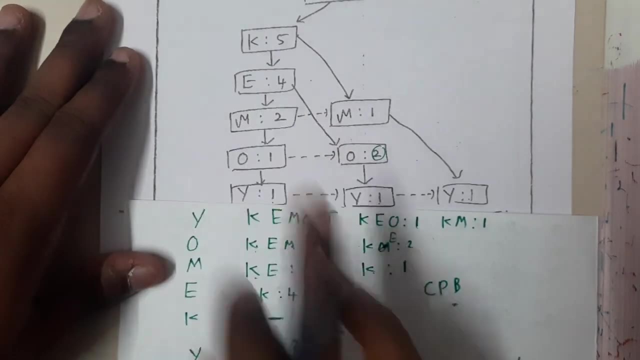 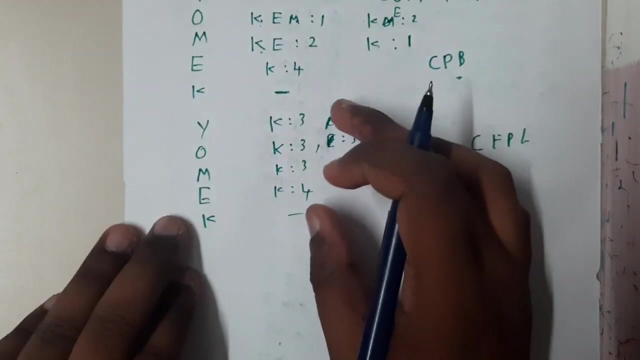 my bad. okay, so it is a k e, guys. it is not k m, yeah, k e to o. okay, exactly, exactly. that's my bad. okay, so k e to okay. so here we got e, okay, done. so now we got these values. so now, based on these values, write all combinational patterns, guys.